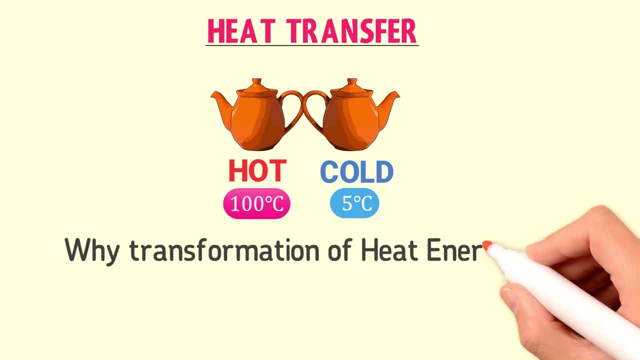 If someone asks you why this transformation of heat energy happens between hot and cold cold objects, the answer is that there is no scientific explanation available behind this transformation of heat energy from hot objects to cold objects. It is a natural process. Heat or thermal energy will transfer from hot object to cold object until both the bodies 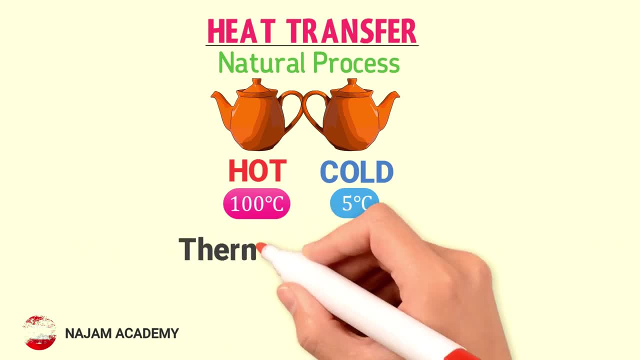 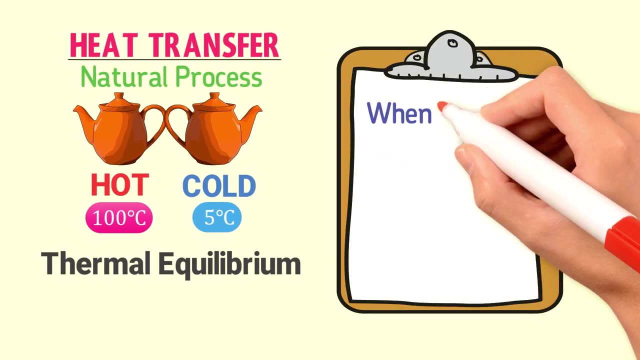 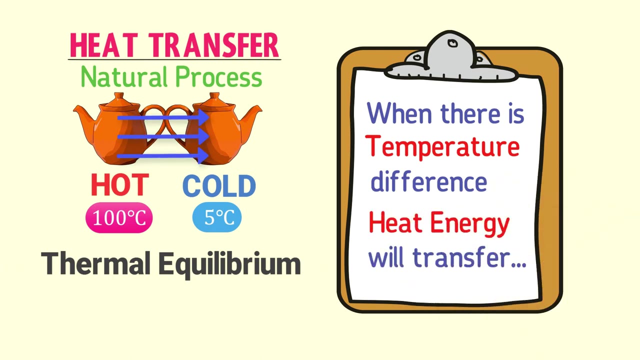 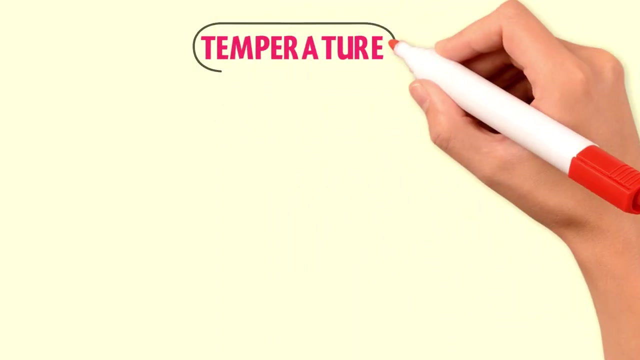 get equal temperature, and this state is known as a thermal equilibrium. You must keep this point in your mind, that whenever there is temperature difference, Heat energy or thermal energy will transfer from hot object to cold object. The second most important concept is temperature. 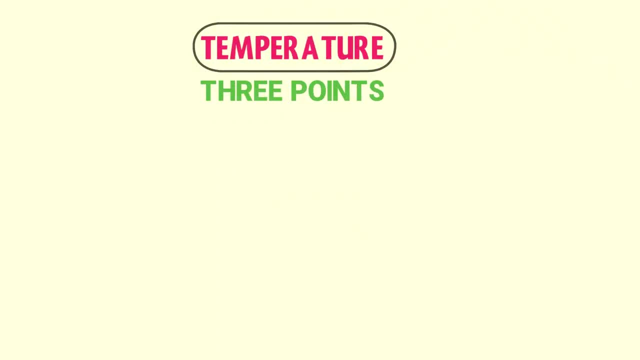 You must know three very important points about temperature in order to learn the first law of thermodynamics. Hence, the first point is that is nothing. It is equal to average translational kinetic energy of gas molecules. In simple words, you can say that temperature depends on average kinetic energy of all the gas molecules present. 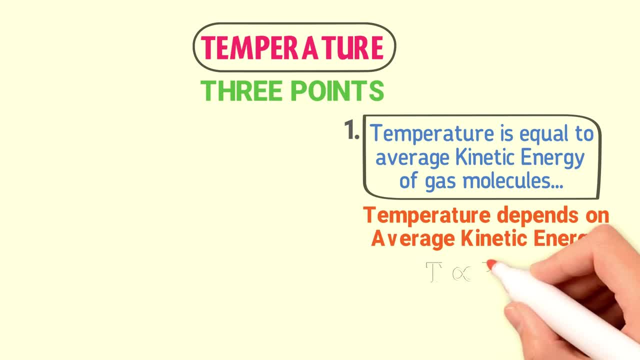 in a system Or you can write: temperature is directly proportional to kinetic energy. If the average translational kinetic energy of gas molecules increases, temperature will also be increased. If the average translational kinetic energy of gas molecules decreases, the temperature of the system will also decrease down. Therefore, the macroscopic form of average. 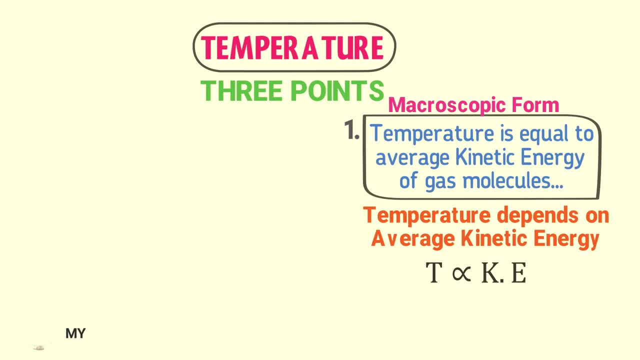 translational kinetic energy of gas molecules is called or termed as temperature. The second important point you should know about temperature is that it measures the degree of hotness or coldness of an object. For instance, if an object possesses large amount of heat or 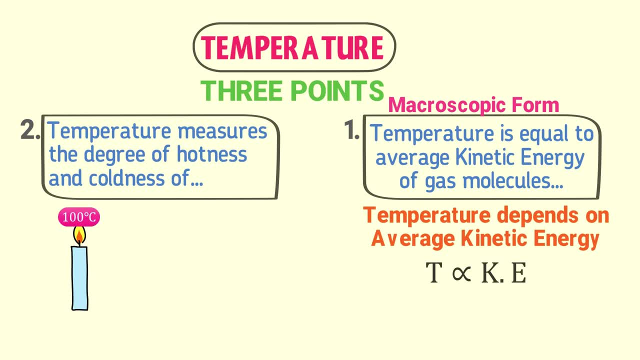 thermal energy, it will be hot and its temperature will be high. Similarly, if an object possesses small amount of heat or thermal energy, it will be cold and its temperature will be high. Thus, the second point regarding temperature is that temperature indicates the amount of heat energy. 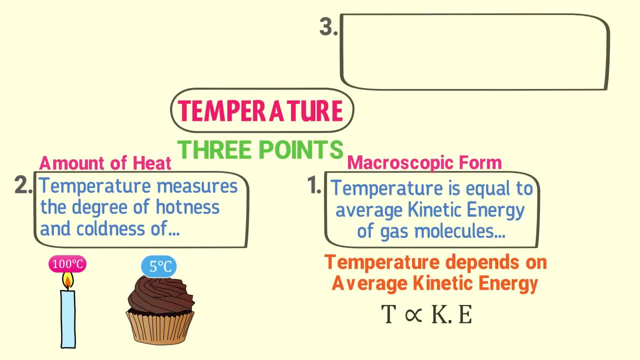 present in an object. The third point about temperature is a bonus point for you or a bonus MCQs. Energy transfer is shown by option A is heat and option B is temperature. Can you guess the correct option? Well, the answer is yes If an object possesses large amount of heat or thermal energy. 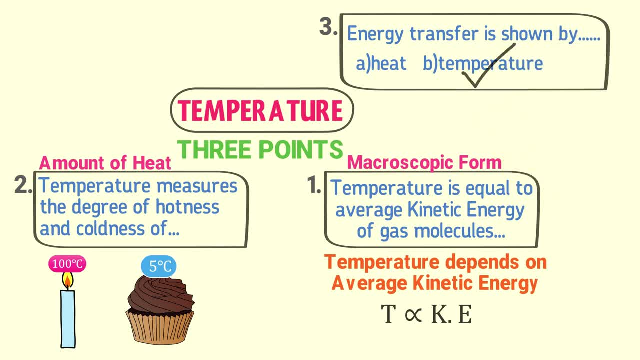 the answer is option B. I mean energy transfer is shown by temperature. The reason is that when an object gets or loses some sort of heat energy, its temperature increases or decreases. Therefore, this increase and decrease of temperature indicates the energy transfer. Now what happens? 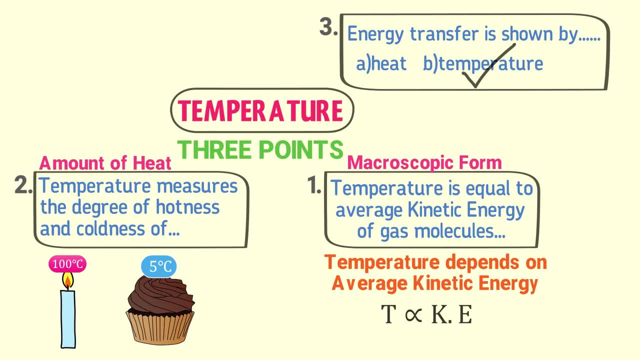 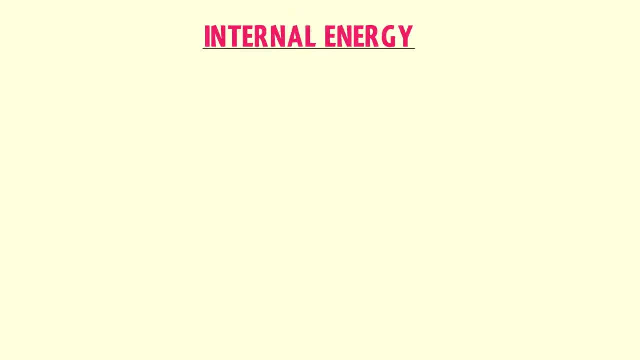 within the body if its temperature decreases or increases. To learn this, you must learn the concept of internal energy. Internal energy is defined as the sum of all forms of molecular energies of a substance. Internal energy is denoted by U. Now, this, all forms of molecular energy, means that gas molecules possess different energies. 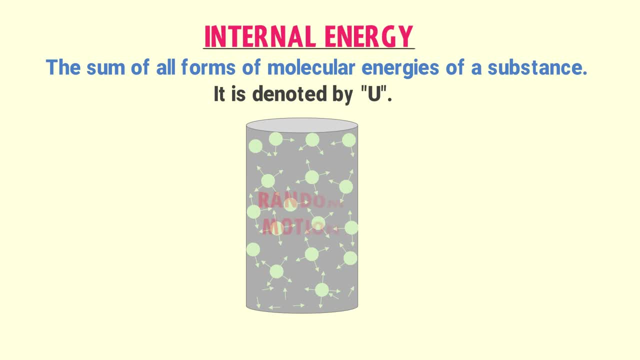 We know that gas molecules are an random motion. When an object is in motion, it possesses kinetic energy. Hence, gas molecules also possesses kinetic energy. Secondly, gas molecules are interacting with each other, due to which they also possess potential energy. Overall, gas molecules possess two types of energy. 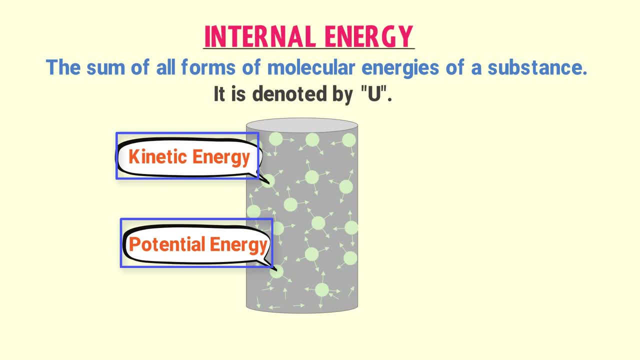 kinetic energy and potential energy. Thus the internal energy of any gaseous system is equal to the sum of kinetic energy plus potential energy. Here let me give you a very important concept quickly. For an ideal gas, the potential energy of molecules are zero. 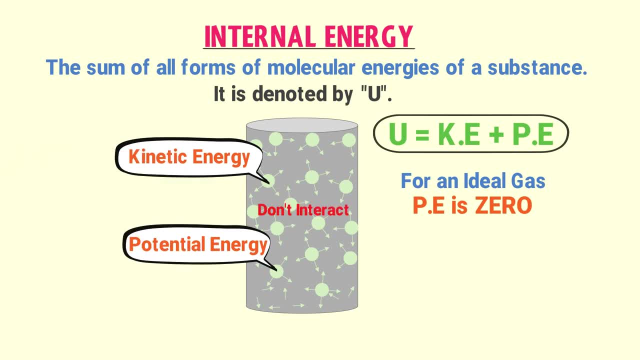 Because we assume that molecules of ideal gas do not interact with each other. they are only in random motion. hence the internal energy of ideal gas U is equal to only kinetic energy, because the potential energy of the gas molecules are zero. Now if we change the kinetic energy of ideal gas as a result, temperature of ideal gas. 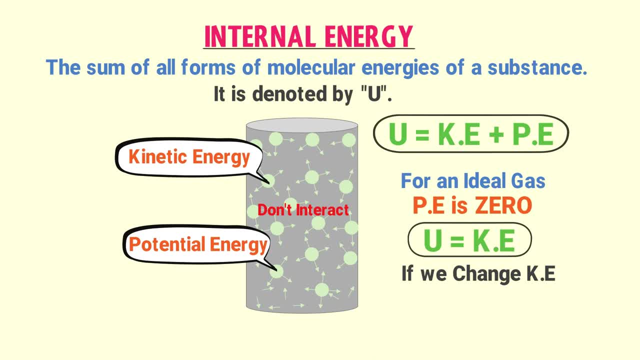 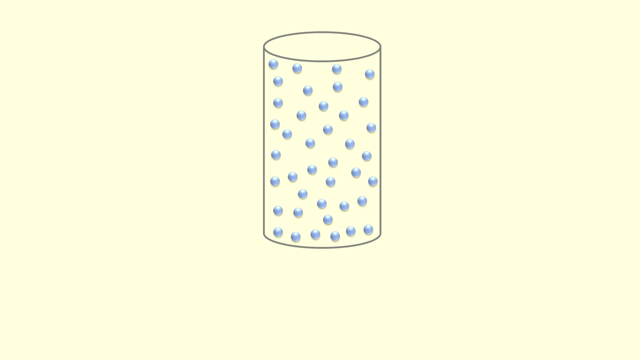 will be changed because there is direct relationship between kinetic energy and temperature, which we assume. Thus, this change in kinetic energy or temperature will change the internal energy U of the ideal gas, For example. consider an ideal gas system. Let the initial internal energy of this gas system is U. 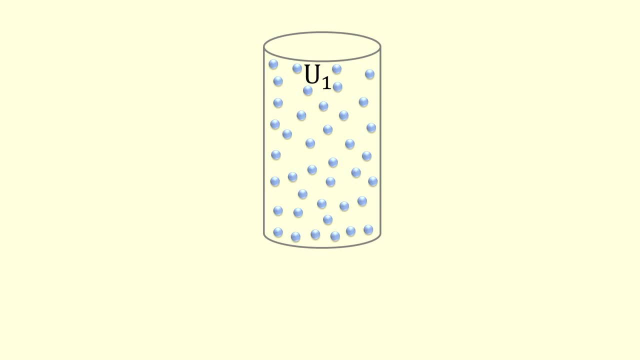 We know that internal energy of an ideal gas is equal to only kinetic energy. hence U1 is equal to U2.. Then if we get this internal energy, U2, it will be equal to the kinetic energy U2.. If we consider N1, we will get the emissions from the gas outside, which will be 1eleri. 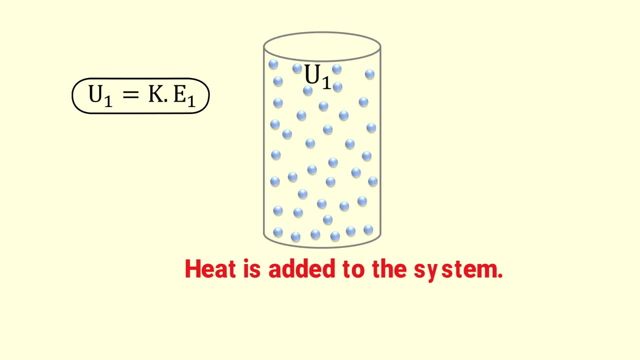 bar propol-1,, which is our thermal energy right now, and N2 is 1, for we just have the total per час. Now use this is pretty normal here. one can get only internal energy and one current method of the gas. 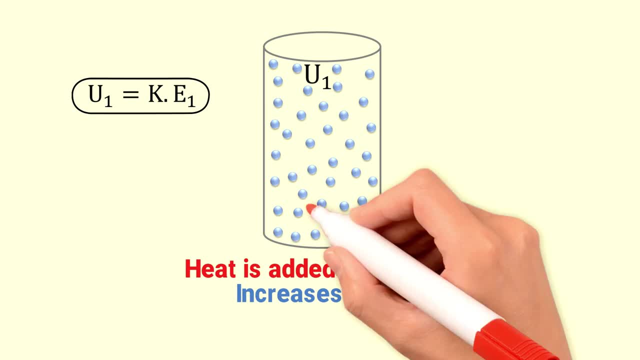 This is definitely the advanced one and still we바 mine. how to get outer energy is with melody at I over here. I percurrent, So fuel is also equal. so right now we take the original temperature of lip. that means the yield does not change the sine. so this is the left, because at this time the internal 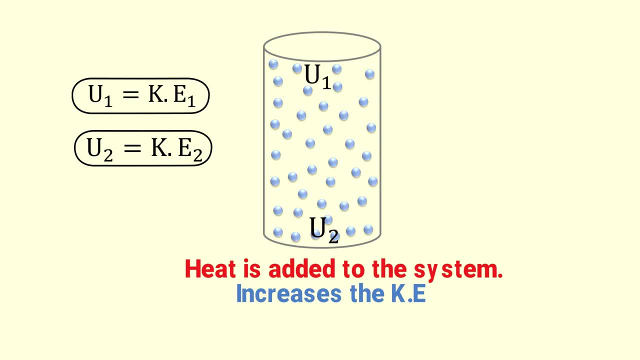 energy will be equal to 1 for the pure kinetic energy. 2. The internal energy of this gaseous system changed from U1 to U2 due to heat Q. This is the central theme of this lecture. If you add some heat Q to a gaseous system, this 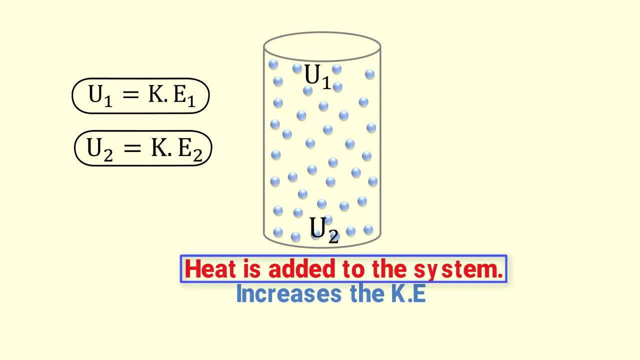 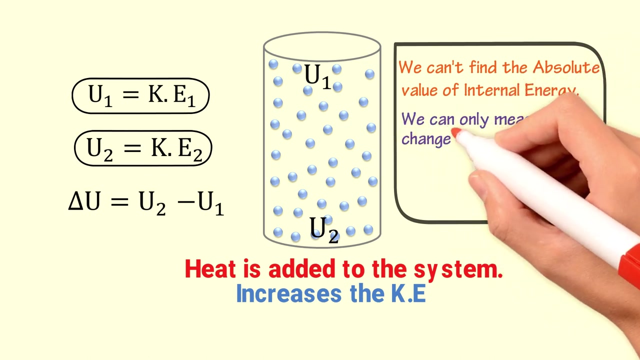 added heat or this addition of heat will change the internal energy of the system. The change in internal energy del U is equal to U2 minus U1.. Remember these important MCQs that we cannot find or measure the absolute internal energy of any system. We can only measure. 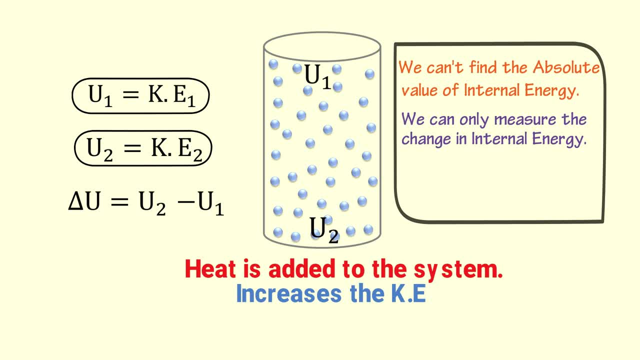 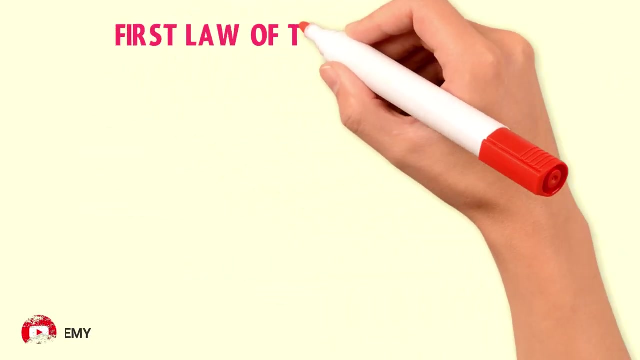 the change in internal energy, because it is a function of state. Secondly, the change in internal energy doesn't depend upon the path. If you have learned all these fundamental concepts, I congratulate you. Now you can learn first law of thermodynamics easily. What is first law of thermodynamics? I always 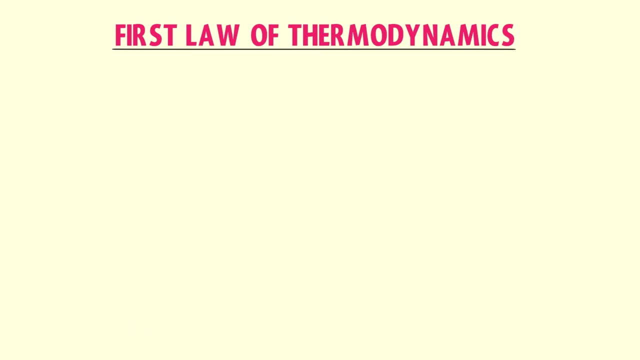 teach it not as first law of thermodynamics. Personally I call it first law of work and heat, because it becomes very easy in this sense. Let's consider gas, in this case closed in the cylinder with a movable, frictionless piston. Let the gas molecules in the cylinder. 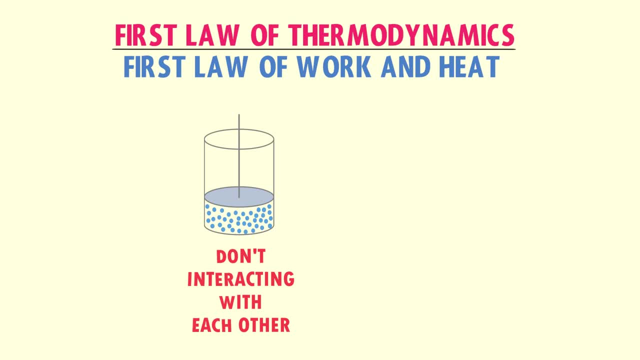 do not interact with each other, Hence their potential energy is zero. The molecules of gas are in random motion, Hence they possess kinetic energy. What about its internal energy U? Well, the internal energy U of this system is: U1 is equal to kinetic energy 1. Now consider: 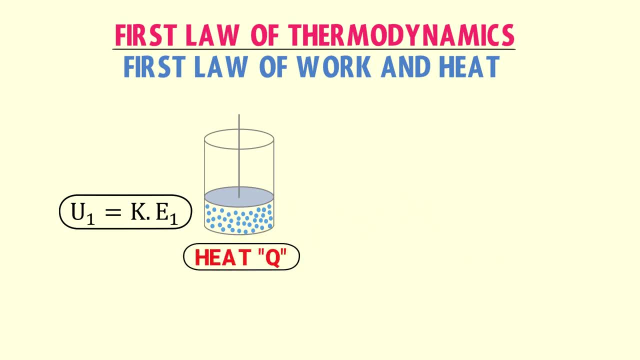 that some sort of heat Q is added to the system. As a result, the movable piston is pushed upward Here. let me ask you a question: What this heat Q is doing. The answer is pretty simple. This heat is doing two important tasks. Firstly, 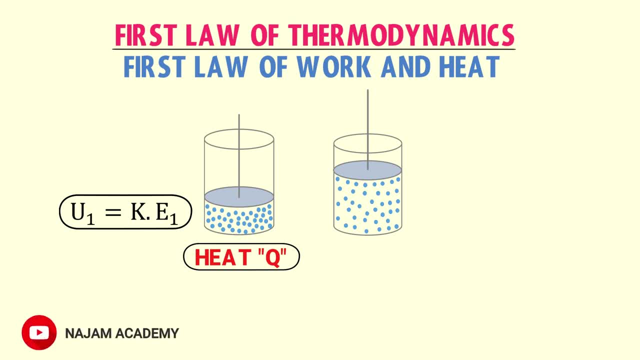 when you add heat Q to this system. as a result, the average kinetic energy of the gas molecules will be increased. When the average kinetic energy increases, both temperature and internal energy will change. Hence this heat Q changed the internal energy of the gas molecule and it becomes: U2 is equal to kinetic energy 2 due to heat Q. Secondly, 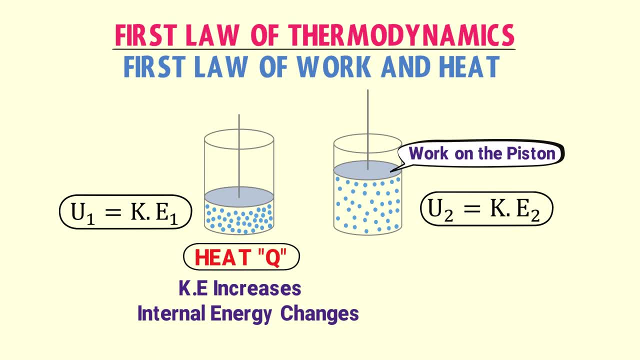 this heat Q has a approximately equal weight, Hence the burning heat Q. there is normal heat. QN does work on the piston. When the gas molecules absorb heat QN, average kinetic energy increases. These molecules rise up and exert force on the piston and upward direction. Hence